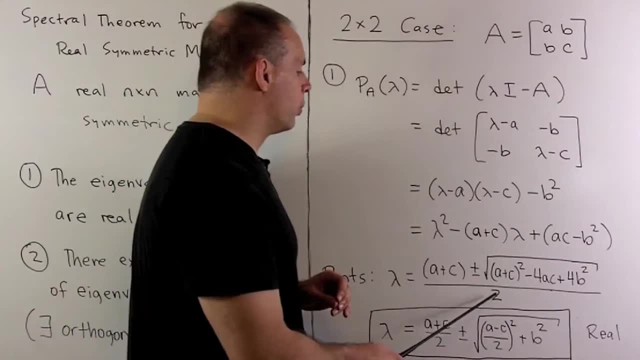 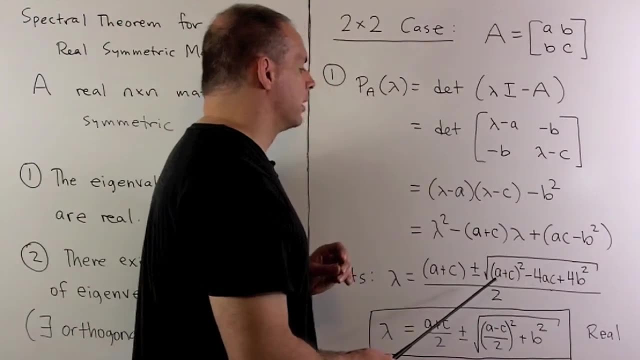 If I want to simplify, well, we'll split this into two terms, So A plus C over 2.. Then over here a few steps. First I'll expand A plus C squared. It gives me A squared plus 2AC plus C squared. 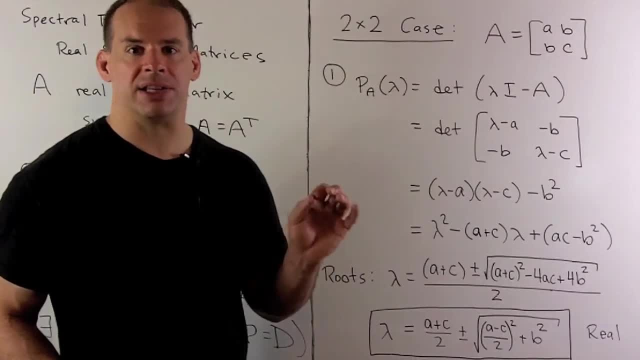 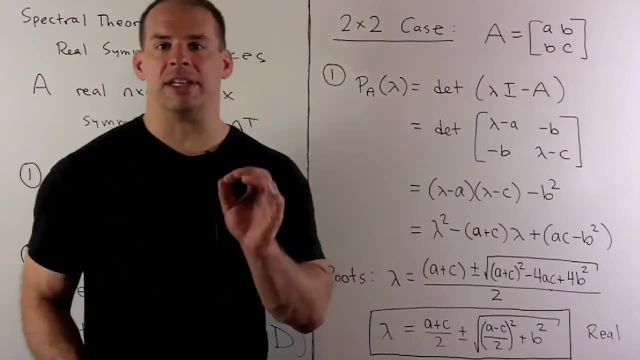 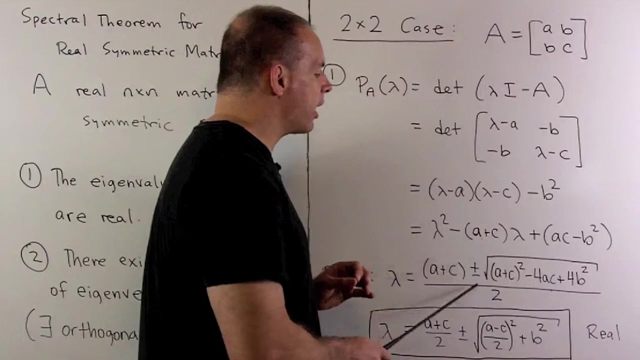 Combine that with the minus 4AC, That becomes A minus C squared. Now if we push this 2 into the square root we'll have a denominator of 4.. For the A minus C squared, I can push that 4 in to the square as A minus C over 2 quantity squared. 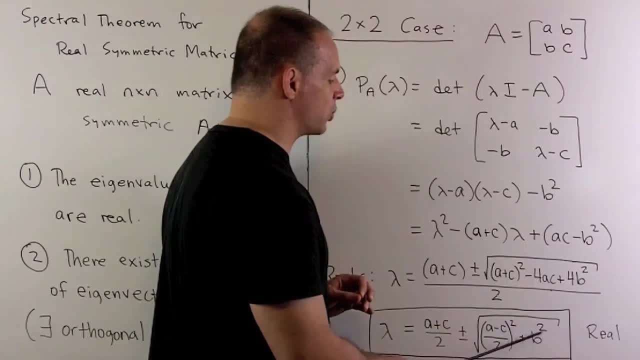 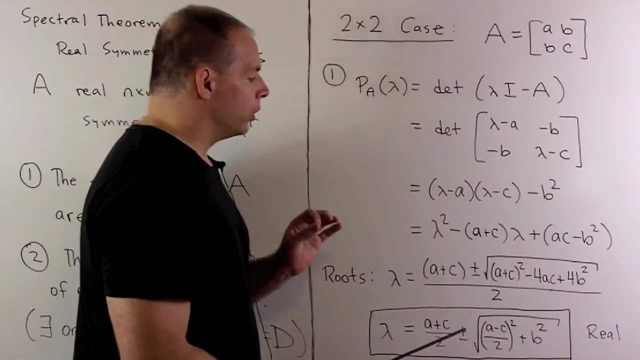 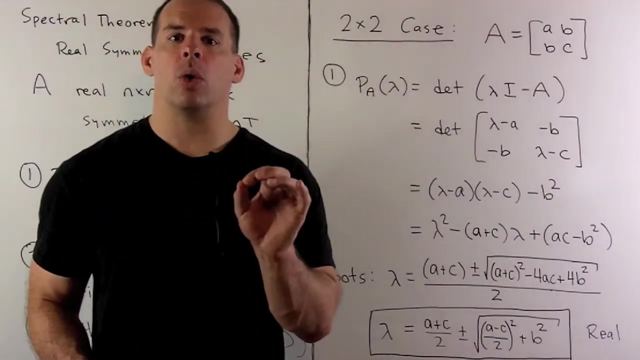 Then when that 4 hits this term, we're just going to have B squared by itself. So here we have our two roots. Now note: we're taking the sum of two squares here. If we take any number and square it, we're going to get either 0 or a positive number. 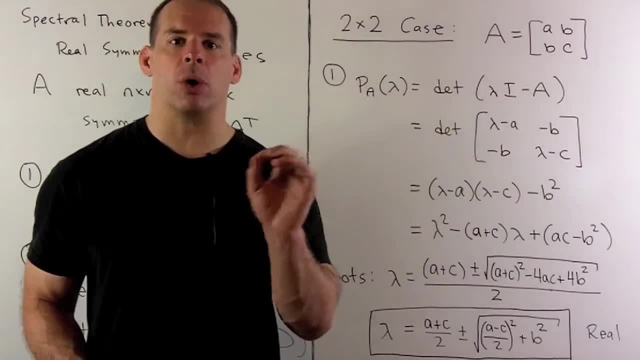 So if we're adding two numbers, we're going to get a positive number. So if we're adding two numbers, we're going to get a positive number. We're going to get two numbers together that are either 0 or a positive. 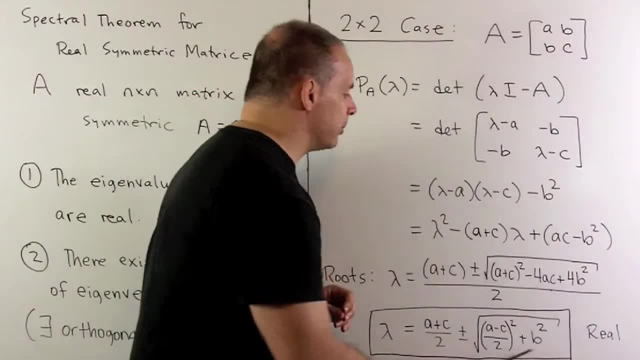 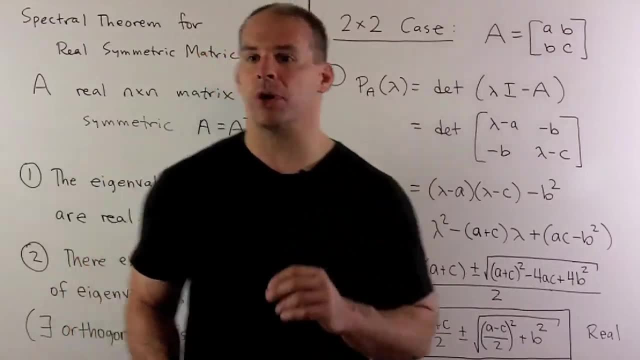 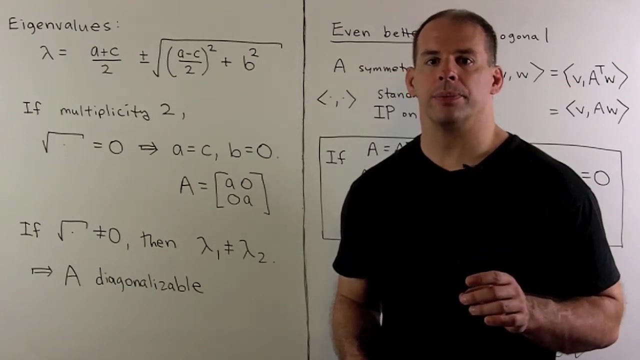 We're going to get another number that's 0 or a positive. So the square root is always going to be a legitimate operation. So that means the roots are always going to be real. And that's our first conclusion. Let's take a closer look at our eigenvalues. 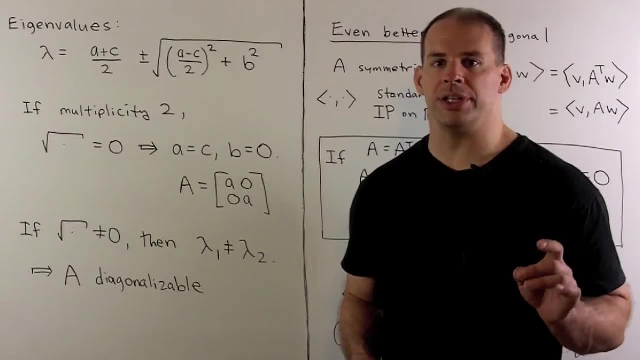 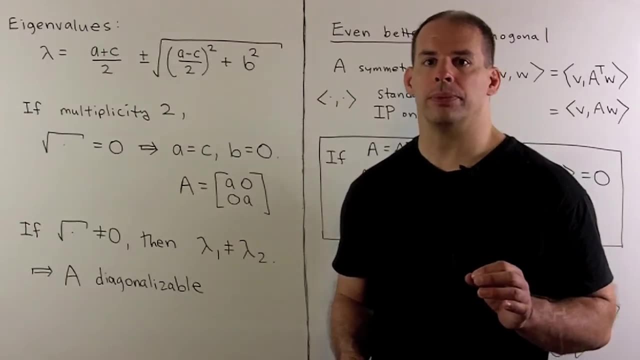 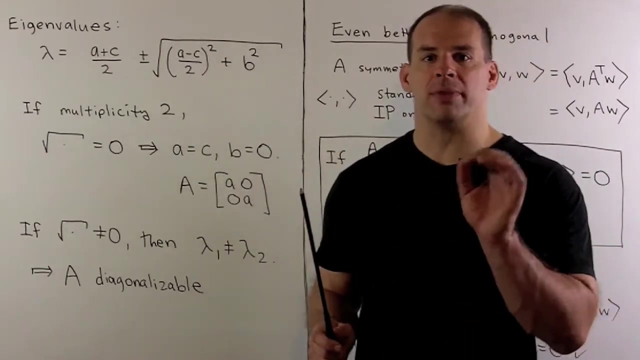 First, we want to know when we have an eigenvalue of multiplicity 2.. That is, when does our characteristic polynomial have a double root? Now, that occurs when the square root is equal to 0. Since we have a sum of two squares that can only be equal to 0 when each item that we're 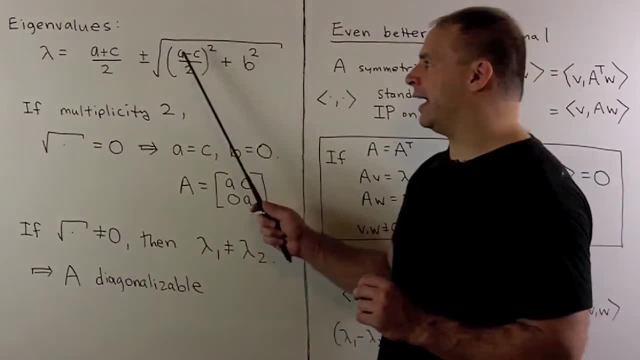 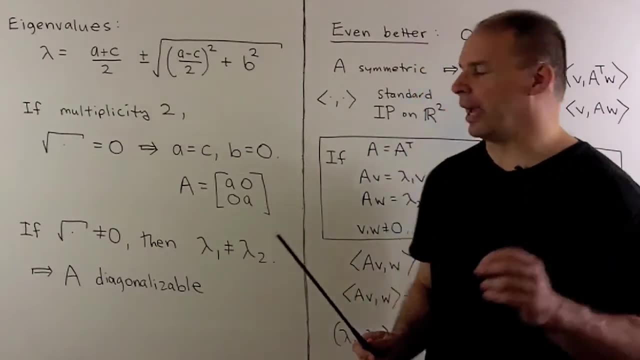 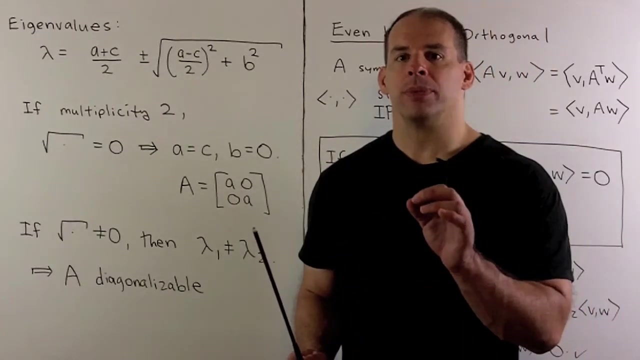 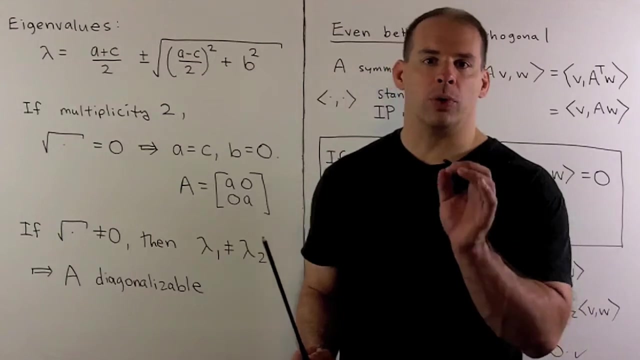 squaring is 0. So we'd have to have A equal to C and B equal to 0. If we put that together, that means our original matrix A is equal to A, 0, 0 A. So the eigenvalues of A are the real numbers, A with multiplicity 2.. For the orthonormal: 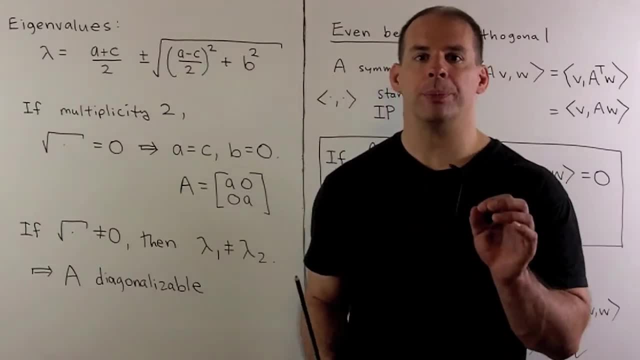 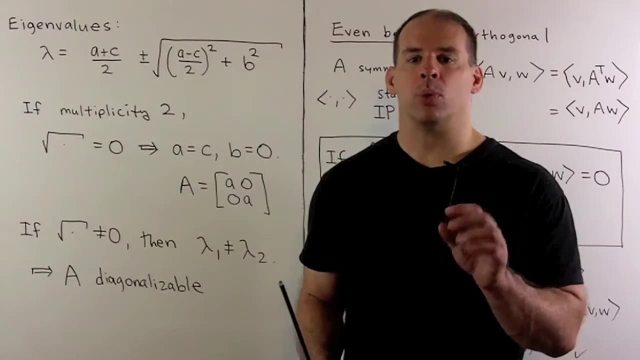 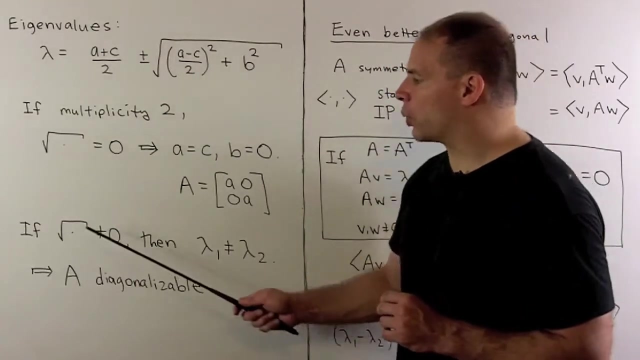 basis. we just use the standard basis E1 and E2.. If we conjugate A by P, which in this case would be the identity matrix, we get back A, which is our real diagonal matrix. Now, if the square root is non-zero, then these two roots are not. 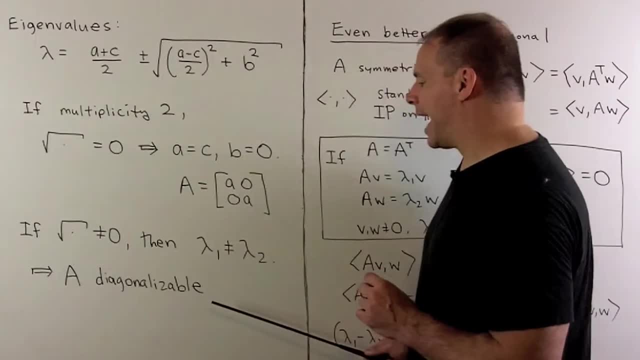 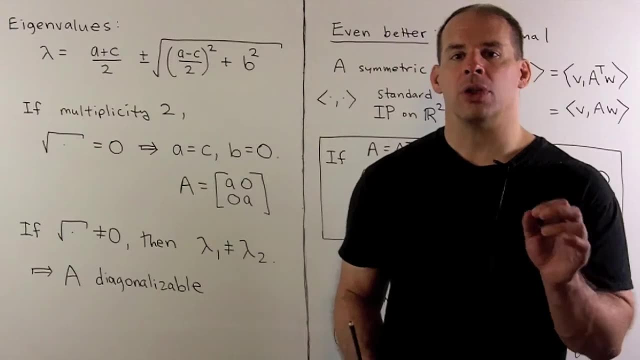 going to be equal to 0. So we're going to have A equal to 0. So we're going to be equal. So A will be diagonalizable. In this case, each eigenvalue produces a non-zero eigenvector. Those eigenvectors are going to be linearly independent, so we'll 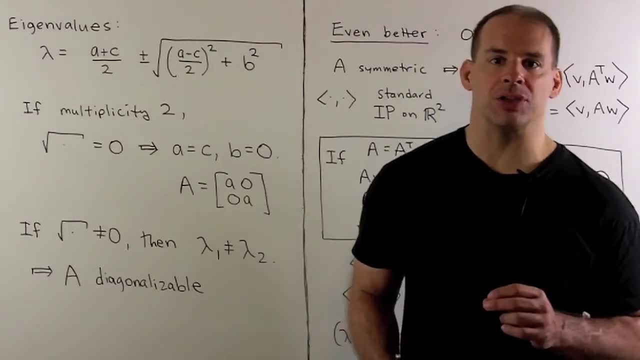 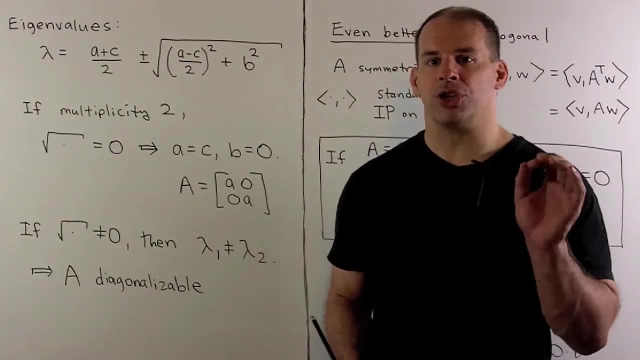 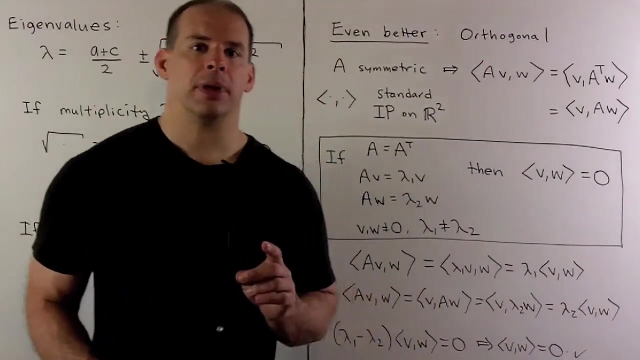 have a basis of eigenvectors, and that's what we need. to be diagonalizable By the spectral theorem, we can do better than that. So the first step is to show that those eigenvectors are actually orthogonal. Now let's review what we have with the standard inner product on R2.. So if A is 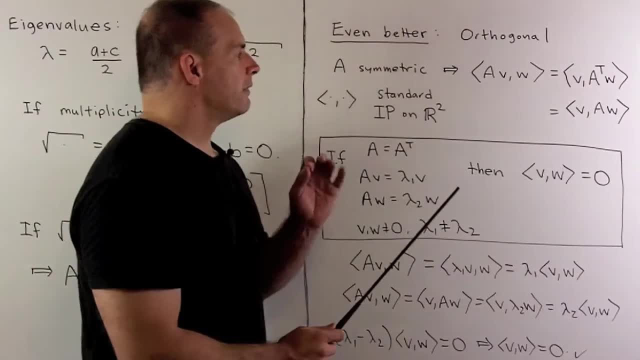 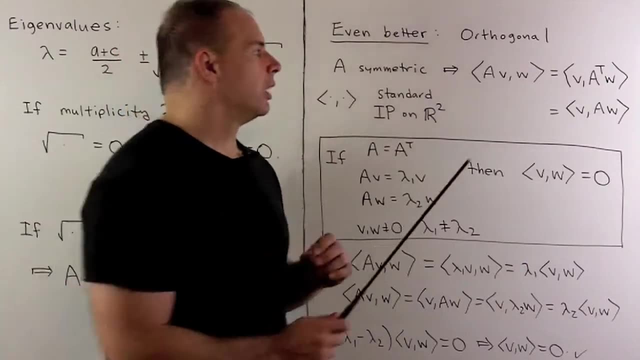 symmetric. we have the standard inner product on R2.. If I take the inner product of A times V with W, the way a matrix works with the inner product, we can push it to the other side by taking the transpose. But because we're symmetric, I'm allowed to remove the. 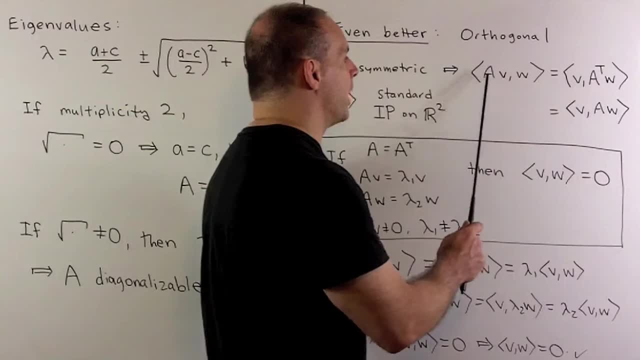 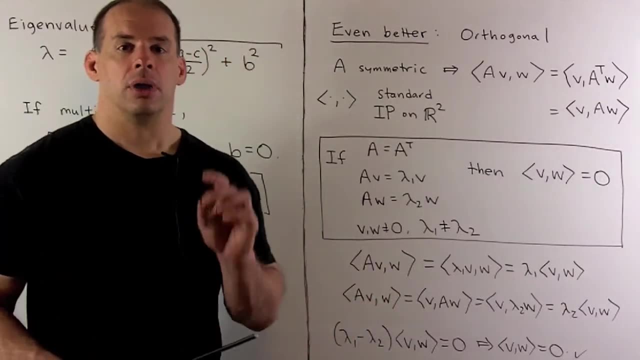 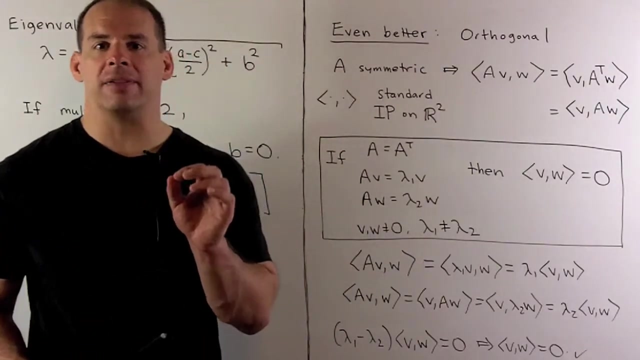 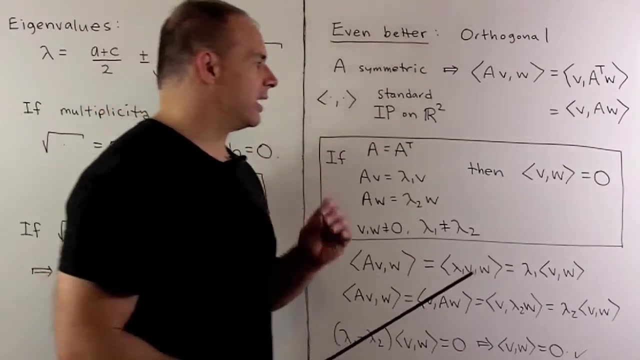 transpose. So if I have a symmetric matrix, I can move our matrix from one side to the other without a penalty. The result we're interested in. if I have a symmetric matrix, we have two non-zero eigenvectors, four distinct eigenvalues, then those eigenvectors are going to be orthogonal. That is we take. 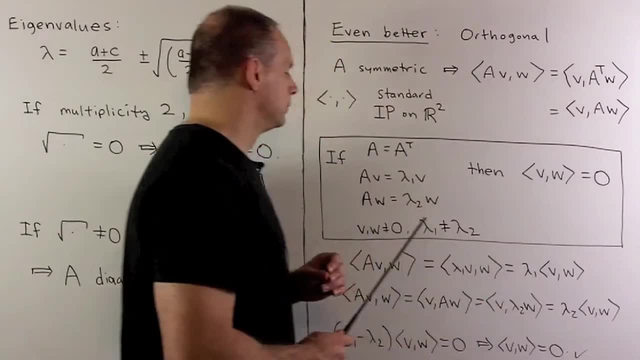 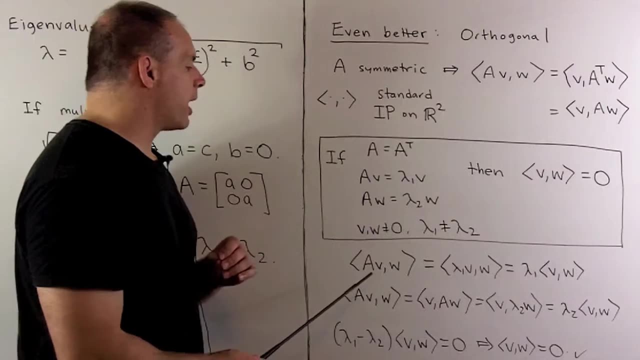 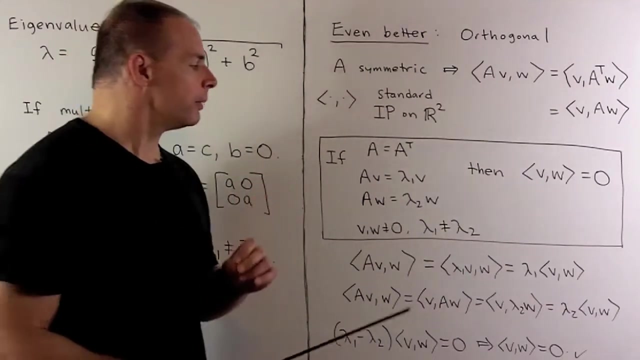 the inner product of V with W, then we get 0.. Now let's just follow our notes and see how it goes and using this result, If we take the inner product of A, V with W, well, A times V is going to be lambda, 1 times V because it's an eigenvector. Then I can pull. 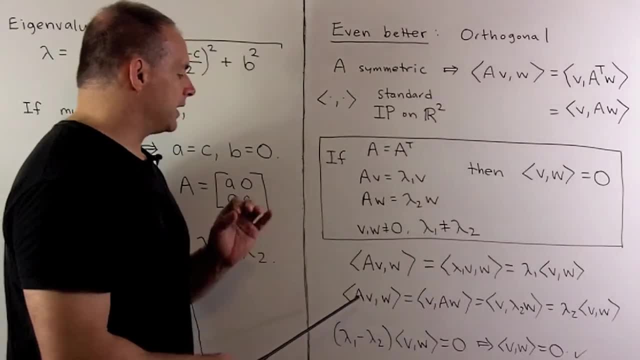 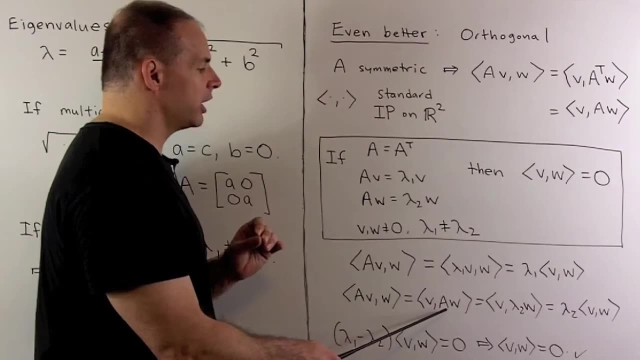 the lambda 1 out in front. If I take the inner product of A, V with W again, instead we'll push the A to the other side as is, because it's symmetric. Then I'll get lambda 2, W. 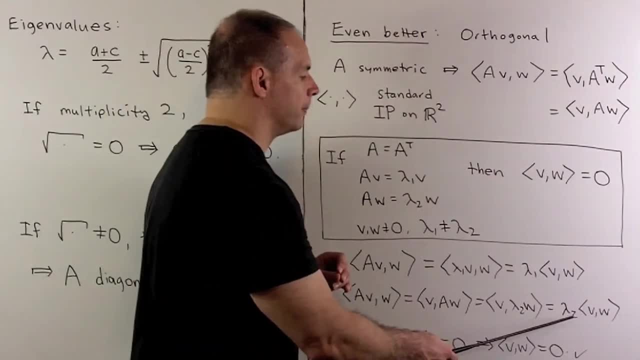 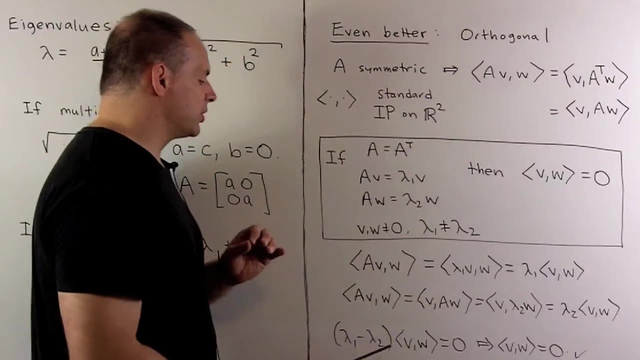 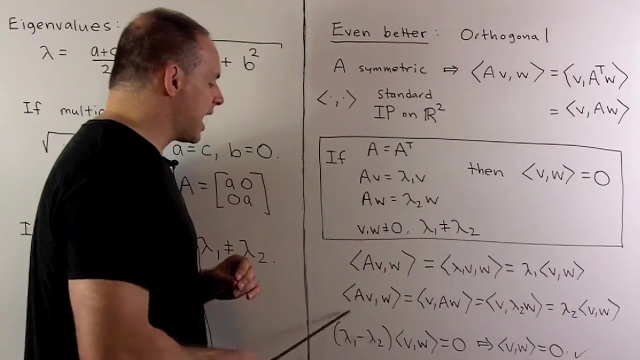 since W is an eigenvector and we can pull the lambda 2 out in front. Now we can push everything to one side, since these are equal. so we'll have lambda 1 minus lambda 2 times the inner product of V and W equals 0. This term out in front is non-zero. 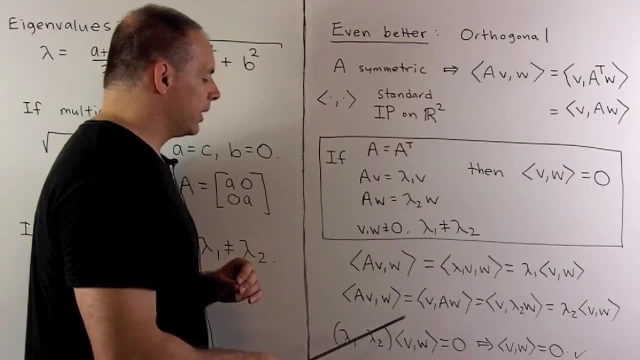 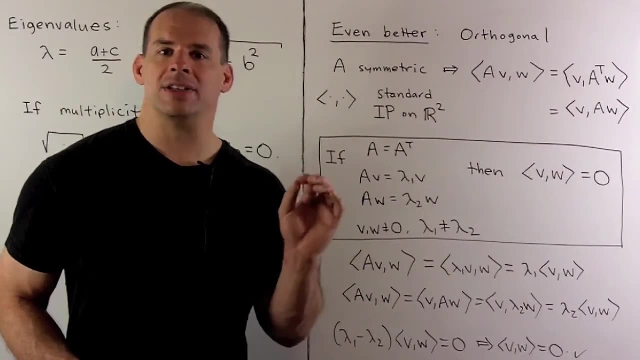 because lambda 1 is not equal to lambda 2, so we can cancel that off. What we're left with is that the inner product of V and W is equal to 0, or V and W are orthogonal, So in this case we'll have: 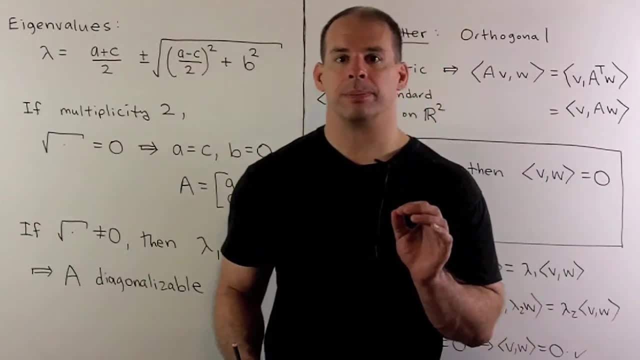 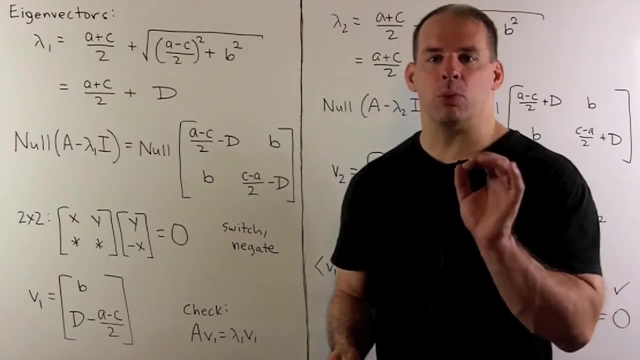 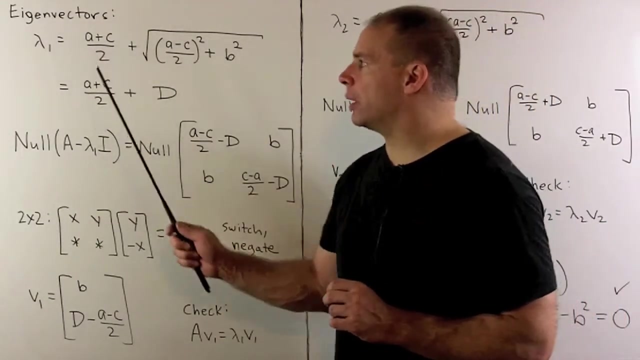 an orthogonal basis of eigenvectors. Now we verify the previous result by finding our eigenvectors concretely and then we'll show that they're orthogonal. We have distinct eigenvalues. so the first one, lambda 1, we're. 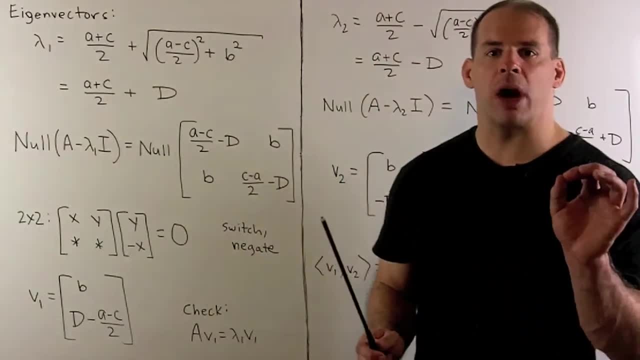 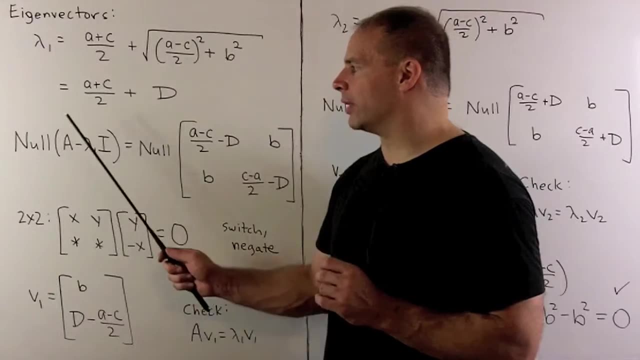 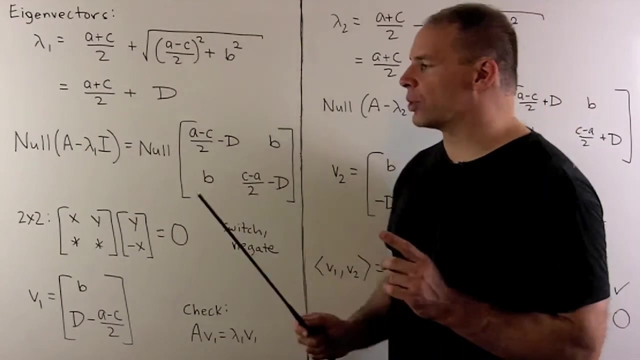 going to use the plus sign on the square root and then for the square root we'll call that D to simplify our notation. To find eigenvectors, we form the null space A minus lambda 1 times I. So we have this matrix here Because we know we have non-zero. 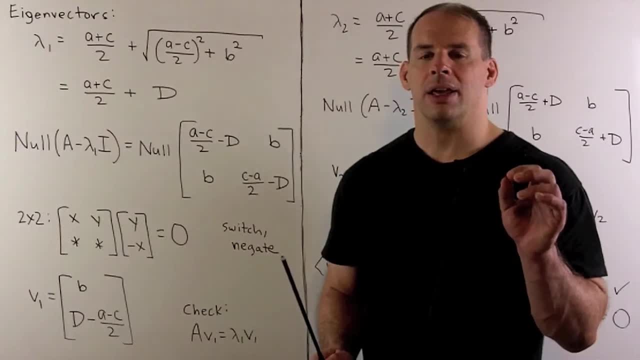 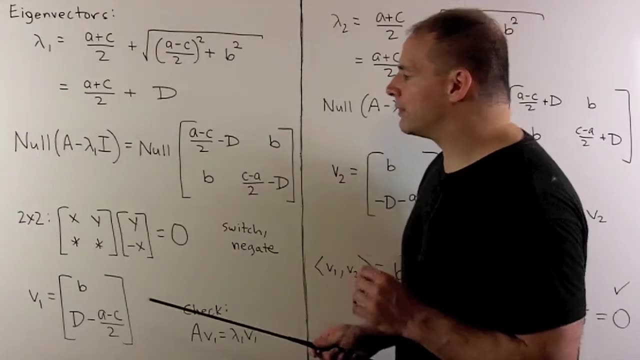 solutions: the determinant is equal to 0.. Now in the 2 by 2 case, if the determinant is equal to 0, we have a trick for finding the null space. I don't have to check the entire matrix, I only need the first row. 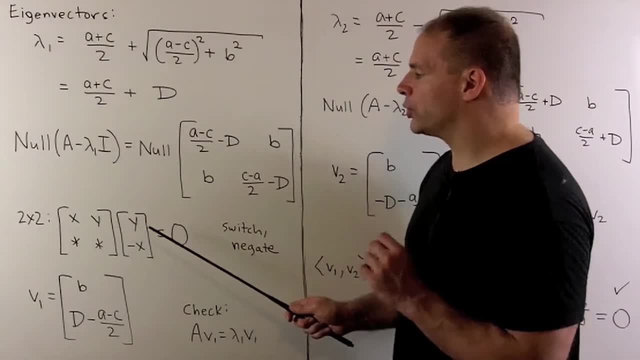 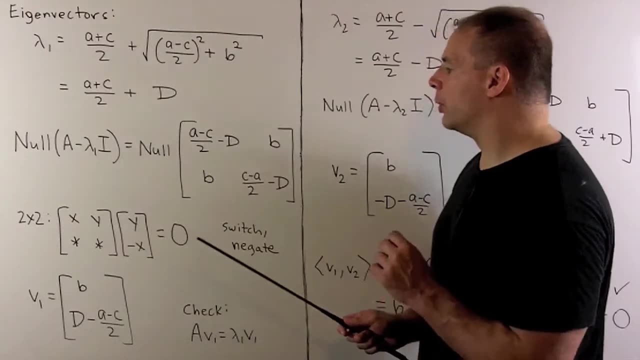 assuming it's non-zero, Then a solution will be to switch these entries and then multiply the second one we're using by a minus sign. So, using this trick, I'll find an eigenvector by just switching these entries and then. 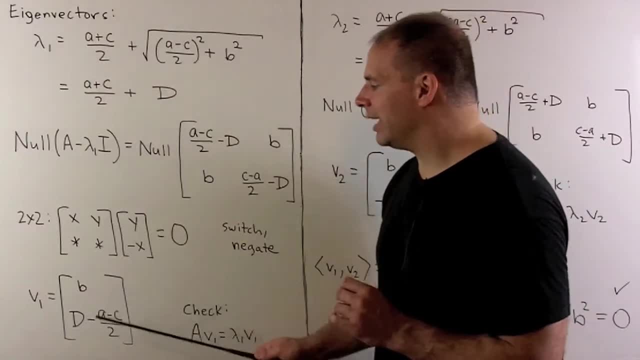 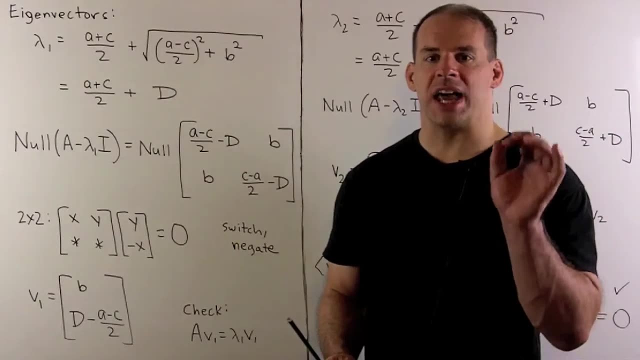 multiplying this one by a minus 1.. So we have B D minus A minus C over 2.. Of course we check that. So if it's an eigenvector for lambda 1, then we have to have the A on. 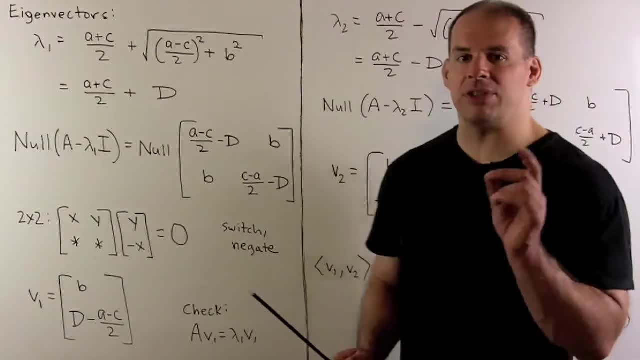 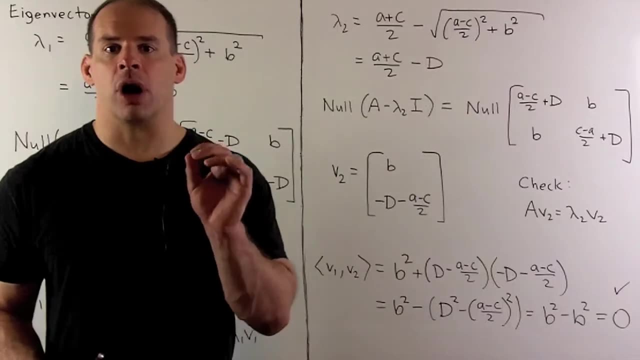 V1 is equal to lambda 1, V1.. So I'll leave it to you to check. That's just an exercise in bookkeeping. Same procedure for our other eigenvalue. So I have lambda 2, we have the minus sign in front of the square root and again I'm 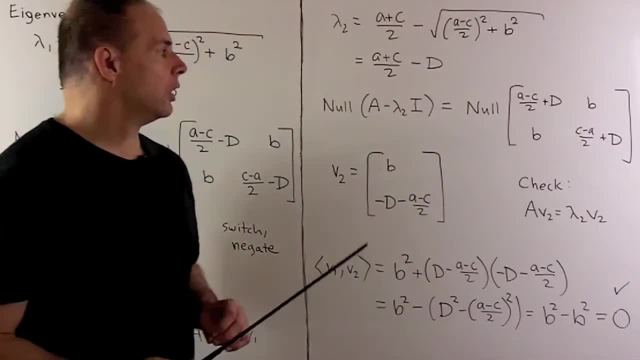 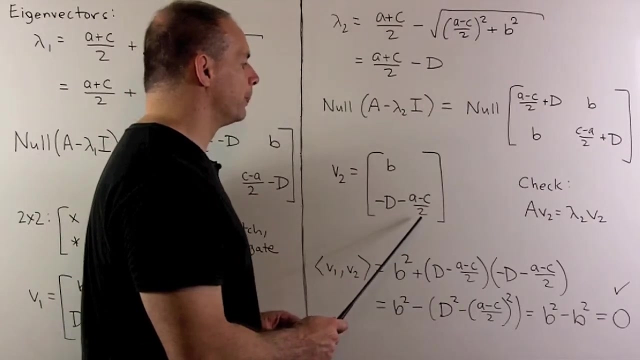 using D to simplify notation. We form the null space, we get this matrix. we apply our trick for 2 by 2 matrices, so we switch and negate. So I get B minus D minus A minus C over 2.. And then I'll leave it to you to check. 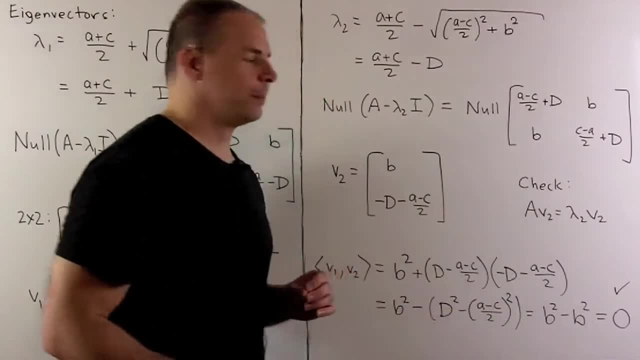 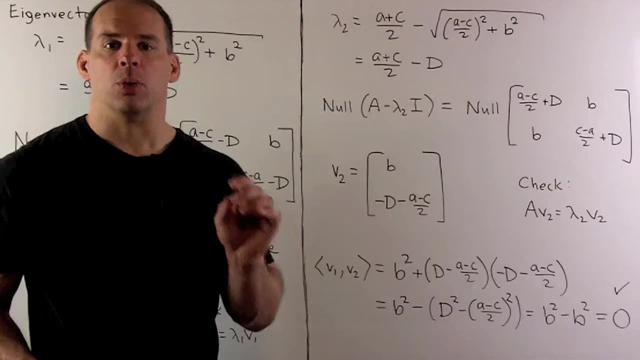 that A on V2 is equal to lambda 2- V2.. So we have our V1 and our V2 eigenvectors for lambda 1 and lambda 2.. We check that they're orthogonal now. So if I take the inner product of V1 and V2,, 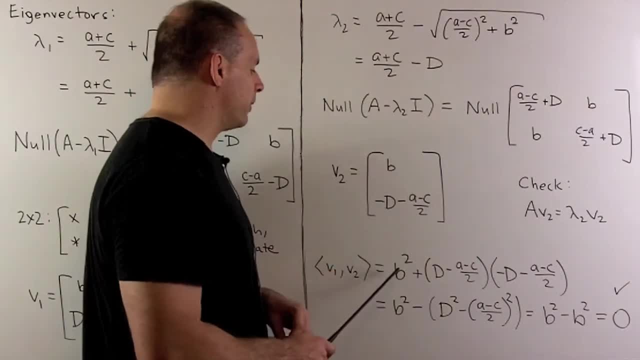 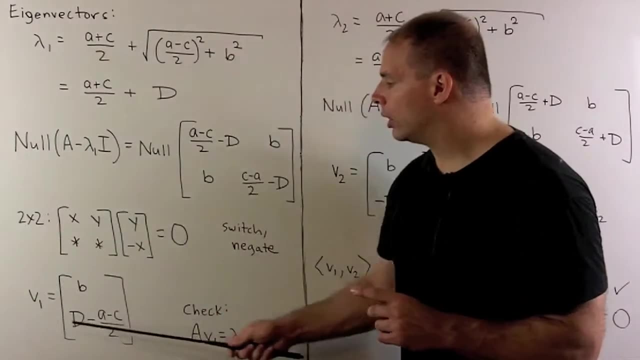 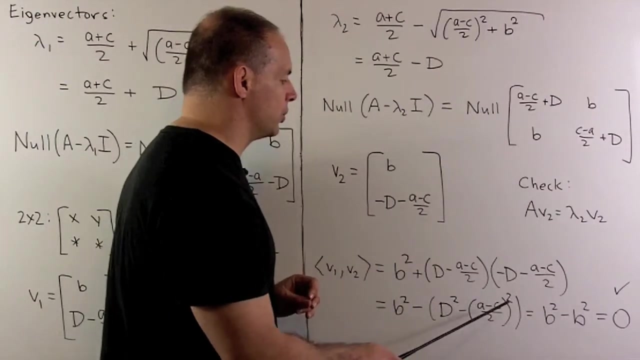 we'll have: okay, both of them start with a B, so I'll have a B squared. Then we note observing each term in the second slot we'll have minus a difference of two squares, So I'll have minus D squared, minus A, minus C over 2 squared. 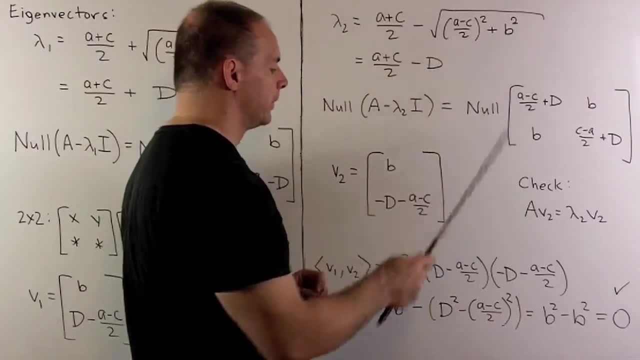 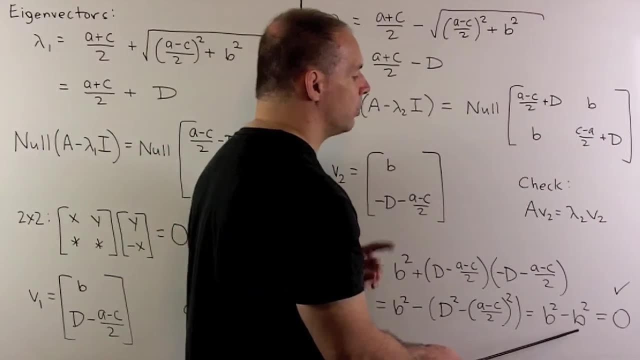 Now when we square D, we're just squaring this term here, so the A minus C over 2 quantity squared is going to go away. I'm going to have B squared minus B squared, which is equal to zero. So these two vectors are orthogonal. 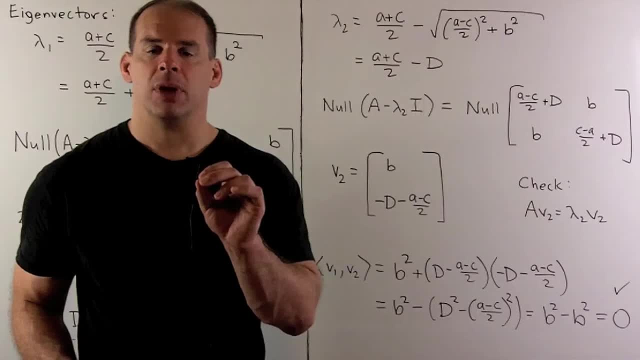 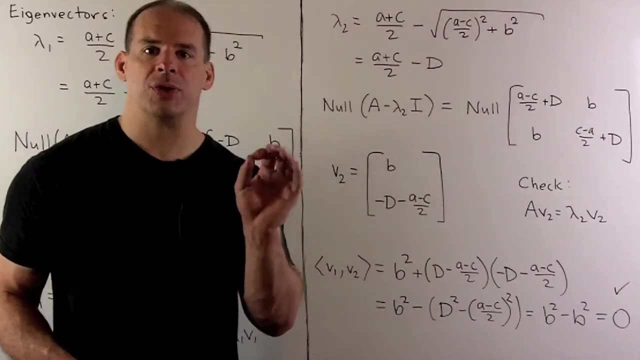 Now, if we want an orthonormal basis, we have to have unit vectors, which would mean we'd have to find the length of each vector and then divide by that length. Of course, here that's going to be messy, so we skip that step. 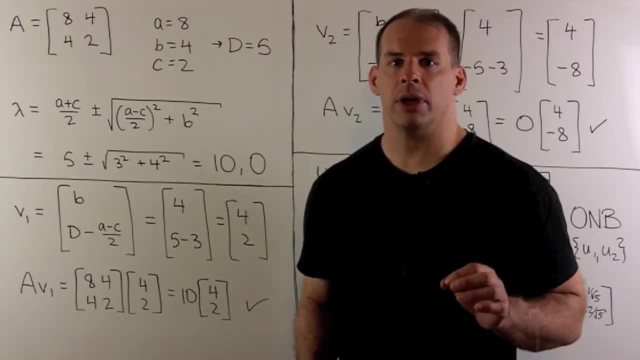 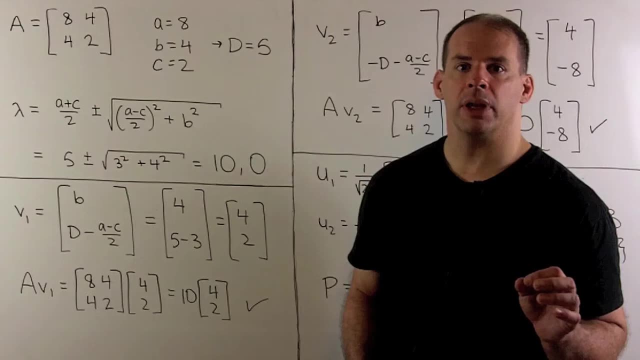 Let's run some numbers through our equations. So we'll use the matrix: A equal to 8,, 4,, 4, 2.. This is real symmetric. We have A equals 8,, B equals 4,, C equals 2.. 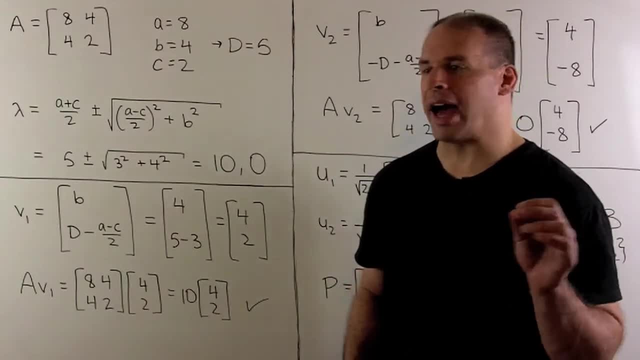 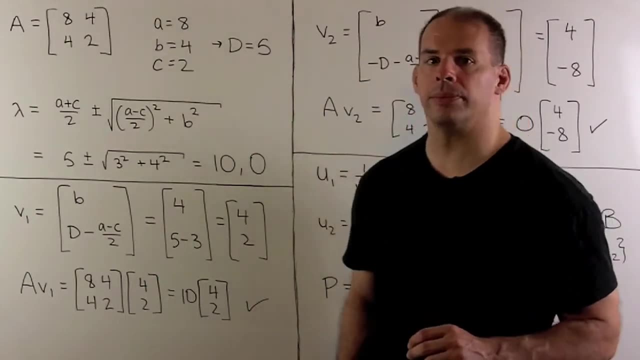 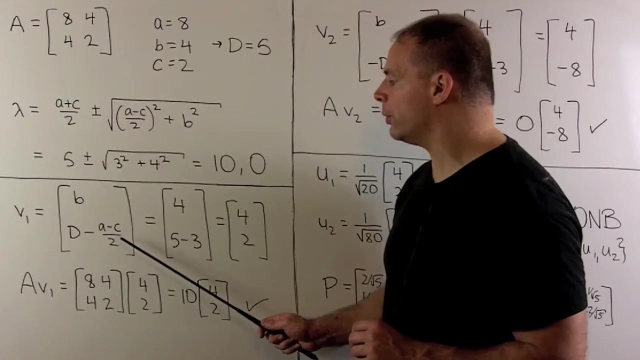 So D is equal to 5.. The eigenvalues are going to be equal to 5 plus or minus 5, which means we have 10 and 0.. Our equation for V1 is: we'll have entries B and D minus A, minus C over 2.. 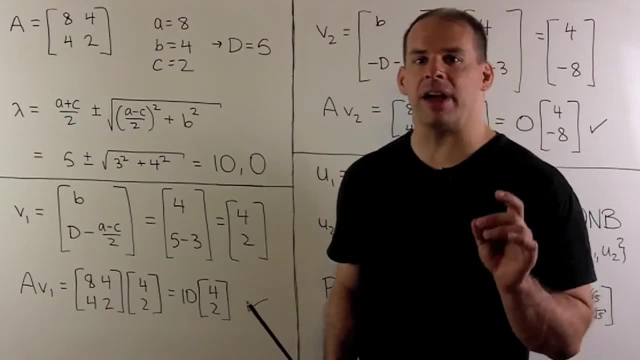 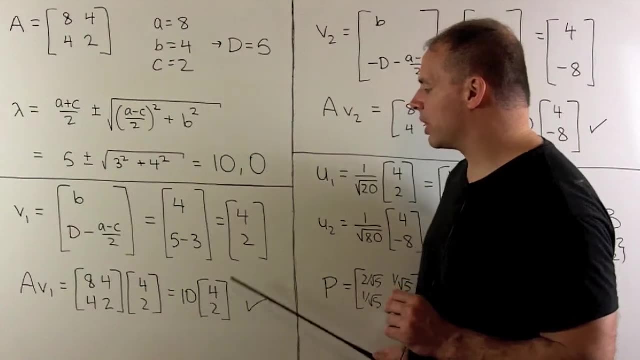 So we'll have 4, 2.. We check that that's an eigenvector, So I'll take A times V1.. We're doing this matrix vector product which gives us 10 times 4, 2.. So 4, 2 is an eigenvector with eigenvalue 10.. 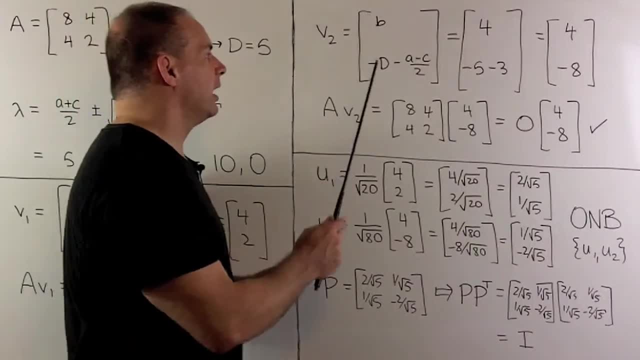 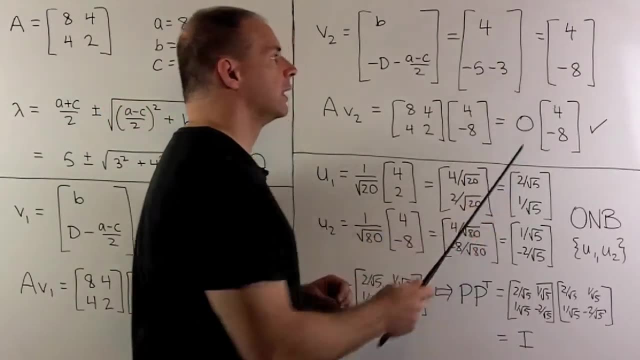 For V2, we have entries B and minus C over 2. So we'll have A minus D minus A minus C over 2. That gives us the vector 4 minus 8.. Again we check, So I'll have A times V2.. 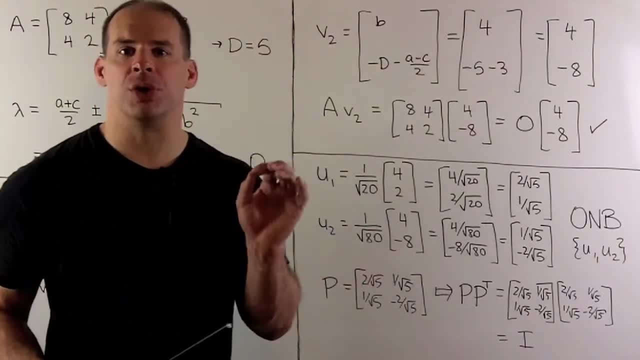 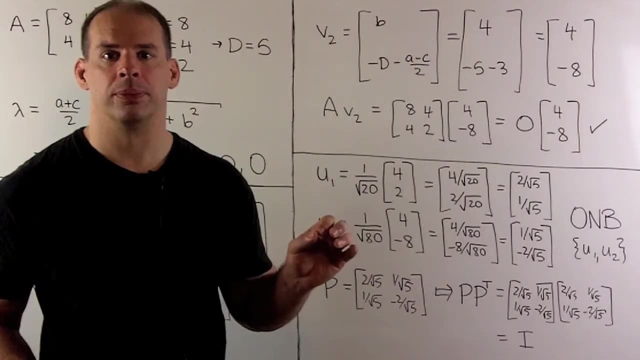 Gives us the 0 vector, which is the same as 0 times 4 minus 8.. So 4 minus 8 is an eigenvector for eigenvalue 0.. Now we check the orthogonal property. So I take the inner product of V1 and V2.. 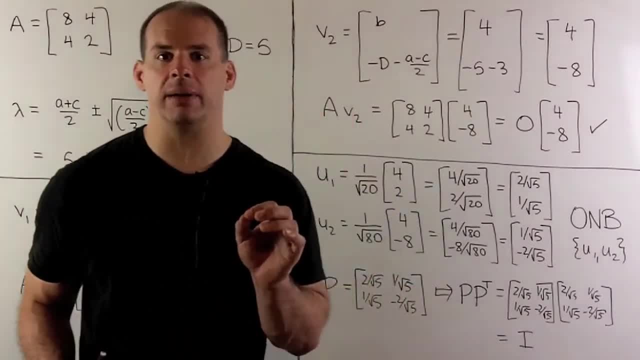 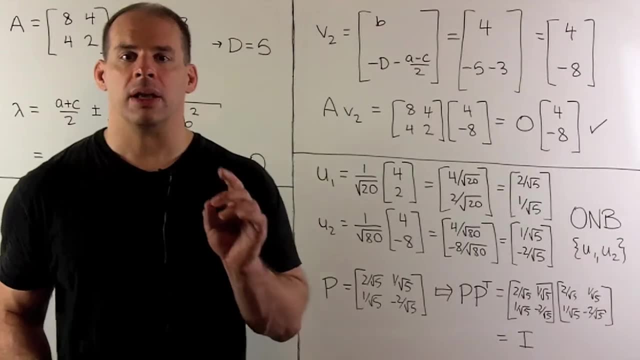 We're taking the inner product of 4, 2 and 4 minus 8. That gives me 16 minus 16,, which is 0. So orthogonal. Now for the spectral theorem. we want an orthonormal basis. 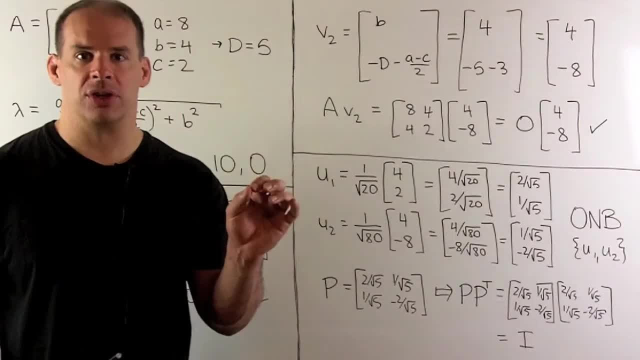 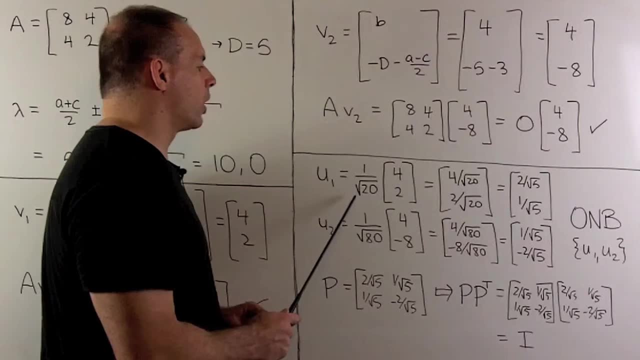 So we'll just take each of our vectors, divide by their lengths. So we want to make unit vectors. So for U1, we'll take V1, divide by its length, which is square root of 20.. For U2, we take V2,. 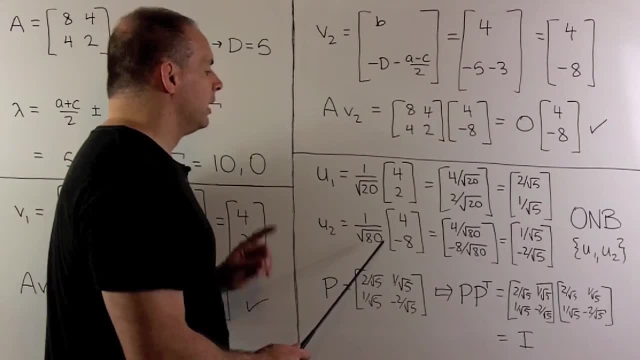 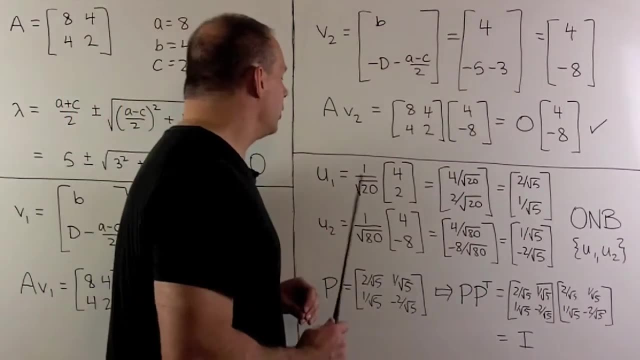 divide by its length, which is square root of 80.. Here I want a nice matrix at the end, So we're going to clean up all our numbers. When I do that, U1 will be equal to 2 over square root of 5,. 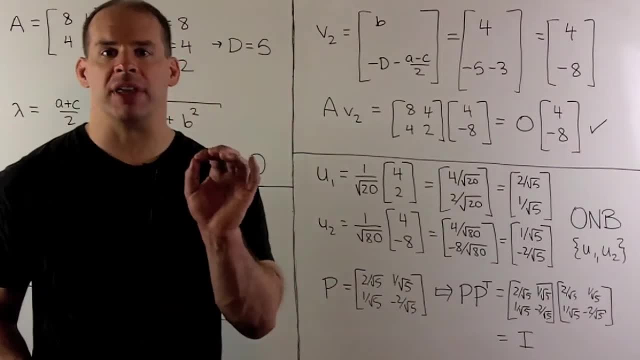 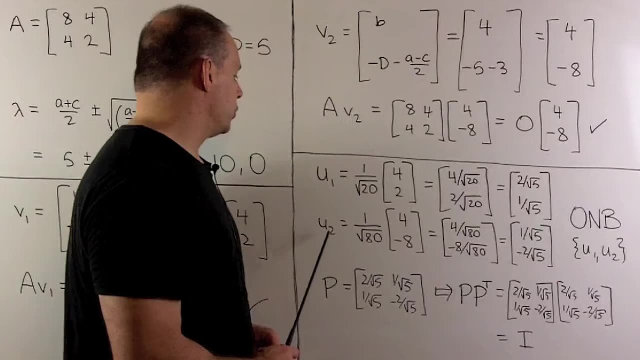 1 over square root of 5.. You sum the squares of the entries. We get 4 fifths plus 1 fifth, So it's a unit vector. Okay, that's a 1.. For U2, we'll have 1 over square root of 5. 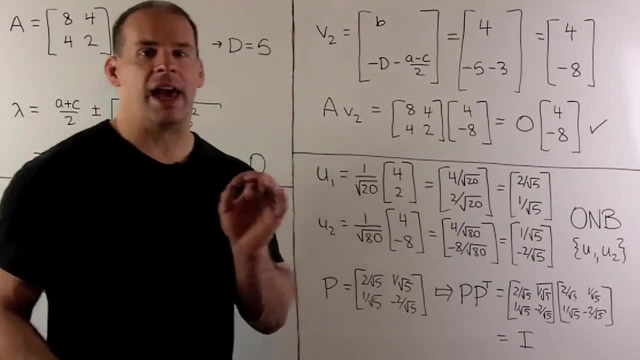 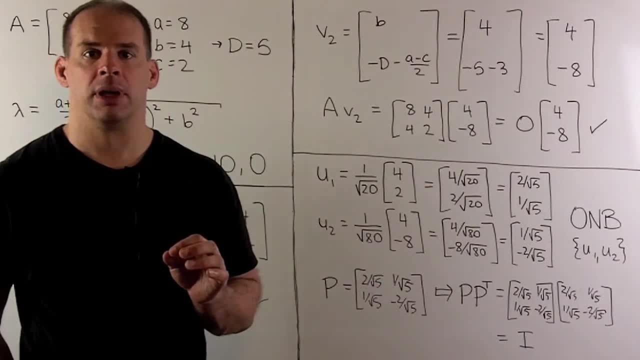 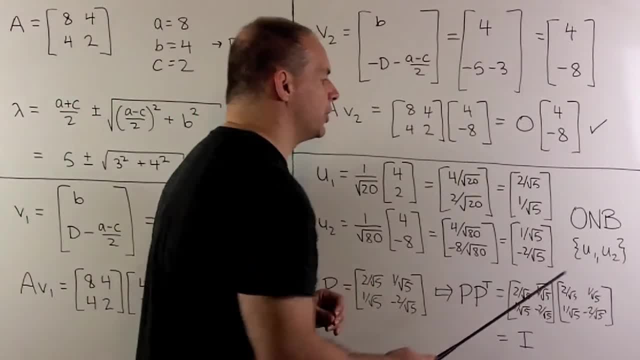 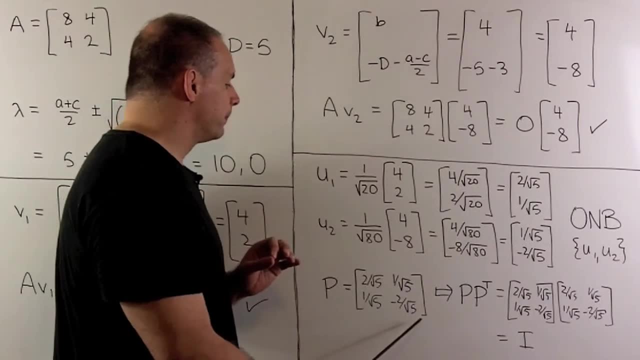 So, to get that, we're going to load U1 and U2 into our matrix P as the column vectors. Now, when we have this, this is going to be an orthogonal matrix, So we want to see that P times P transpose. 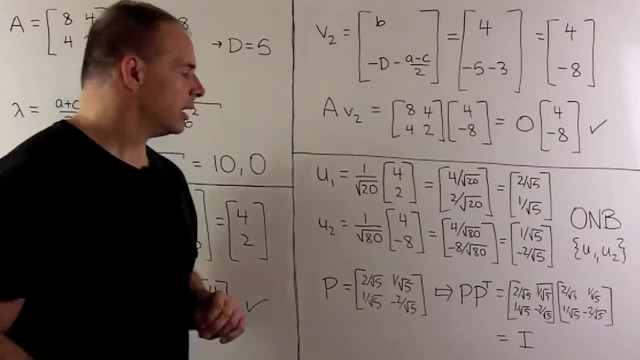 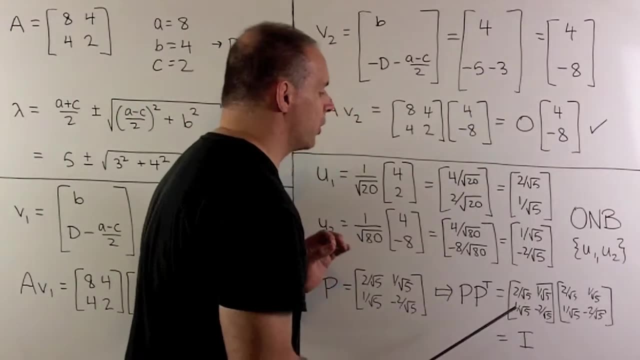 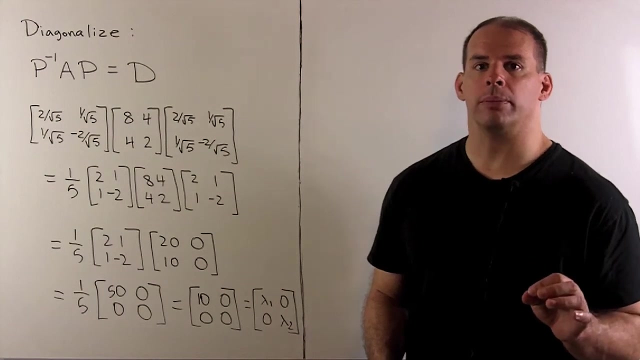 gives us the identity matrix. In this case, P transpose is just equal to P, So I'll leave it to you to do the multiplications here that show that we get the identity. To finish, let's put our matrix in diagonal form. 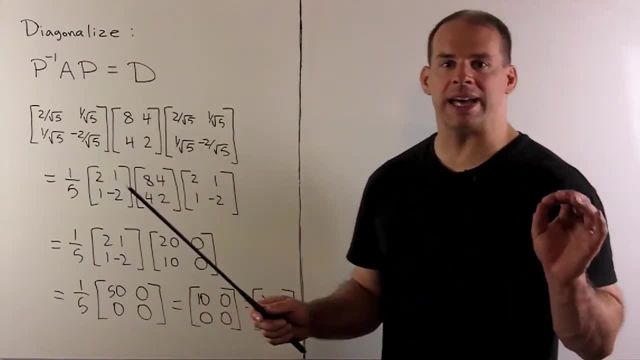 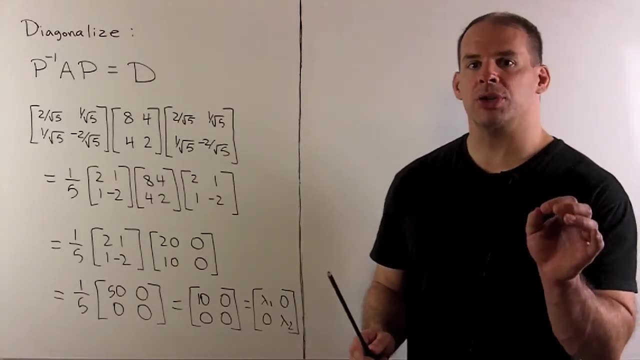 So we'll form P, inverse A P and show that we get a diagonal matrix out. and show that we get a diagonal matrix out. Now, P is going to be the matrix where the columns are our eigenvectors, D is going to be a diagonal matrix. 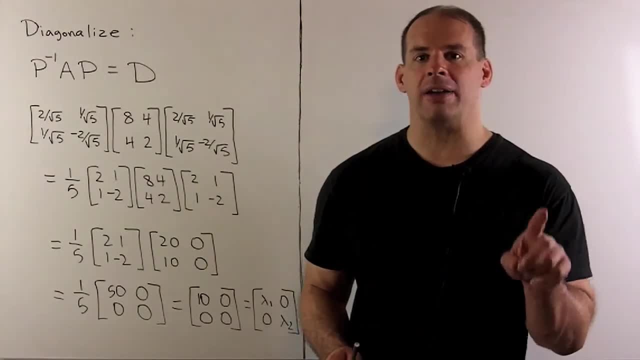 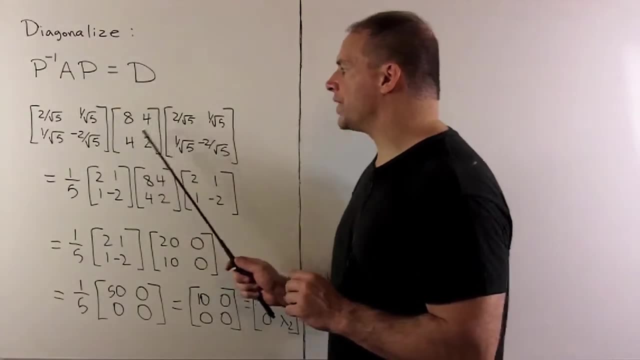 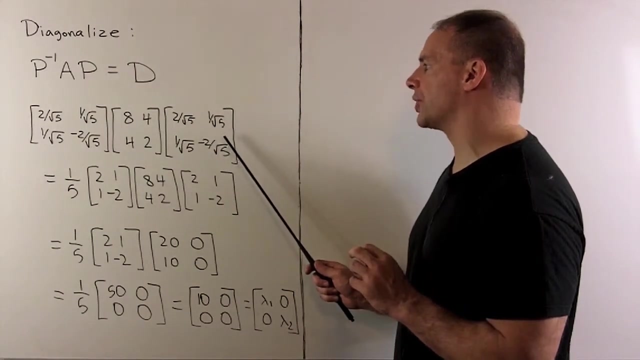 with the eigenvalues on the diagonal. Here the eigenvectors and eigenvalues go in the same order, So we'll form P inverse A P. Here we have that P inverse is equal to P transpose, which just happens to be equal to P also. 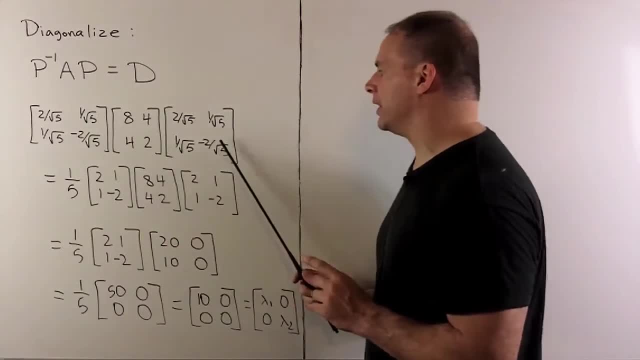 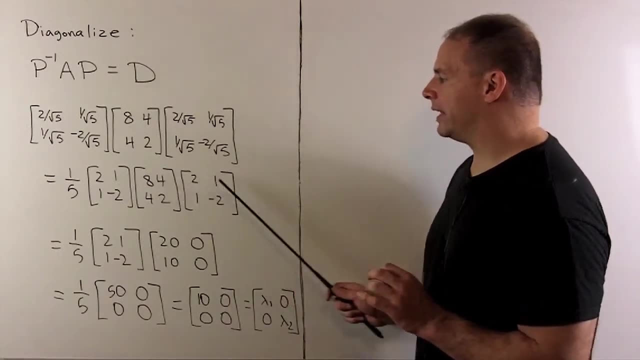 I could pull 1 over square root of 5 out of each of these matrices to give us a one-fifth out in front, and then these are easier to look at. We multiply these two matrices together and we get 20, 0,, 10, 0.. 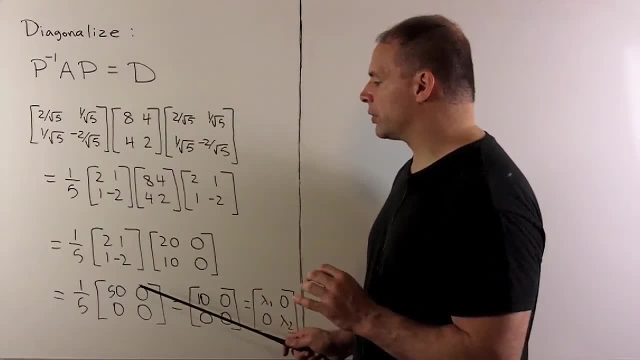 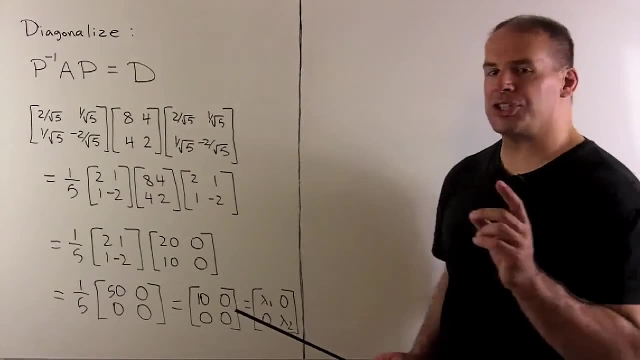 Then if I take this product, I wind up with 50, 0, 0, 0.. We multiply by one-fifth, I get 10, 0, 0, 0. And that's just the diagonal matrix. 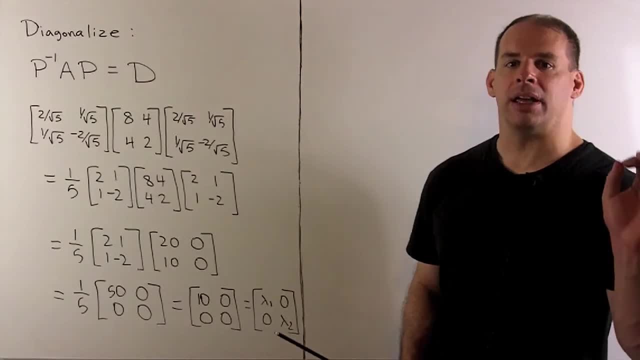 with our eigenvalues of 10 and 0 on the diagonal, in the same order as our eigenvectors. 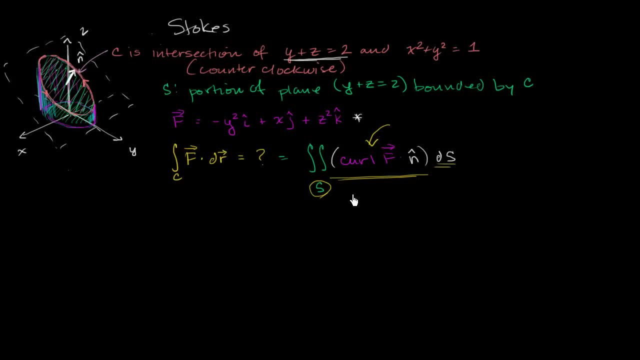 Now that we've set up our surface integral, we can attempt to parameterize the surface, And one way to think about it is we want our x and y values to take on all of the values inside of the unit circle. what I'm shading in right over here: